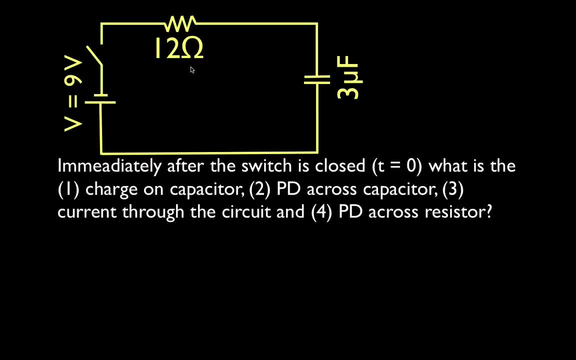 this is the circuit we're going to use for this video. We have a 12-ohm resistor, a 3 microfarad capacitor and we have a 9-volt power supply, And we're going to look at this circuit in two different time zones, two different times. One is immediately after the switch. 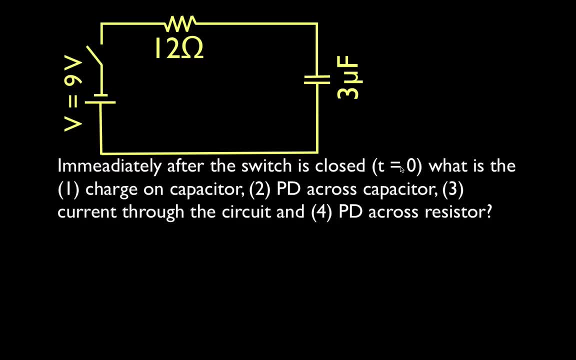 has been closed, which we often call time equals zero. Now, I think of it not really as time equals zero. It's right after the switch has been closed, so it's not really zero, It's a fraction of a second or a very small amount of time. 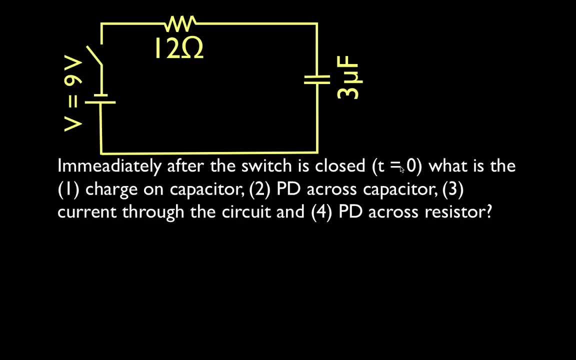 But what happens? what does this circuit look like right after the switch has been closed? We want to know what is the charge on the capacitor, what is the potential difference across the capacitor, what is the current through the circuit and the resistor and 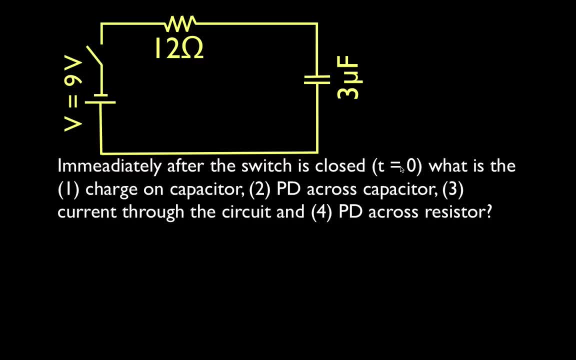 what is the potential difference? or the voltage drop across the resistor. And this is right after the switch has been closed. And this is the way I think about this type of problem: Right after the switch is closed, all of the current, the total amount of current, the 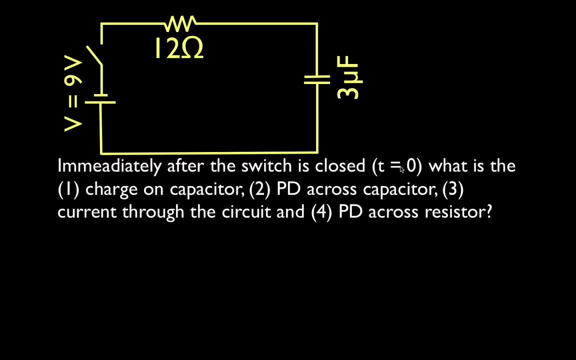 current is flowing through the circuit and the resistor, But none of this current or no charge has yet reached, or no charge has been put onto the capacitor. There is no charge on the capacitor. Okay, None of the charge has reached the capacitor, So really right. 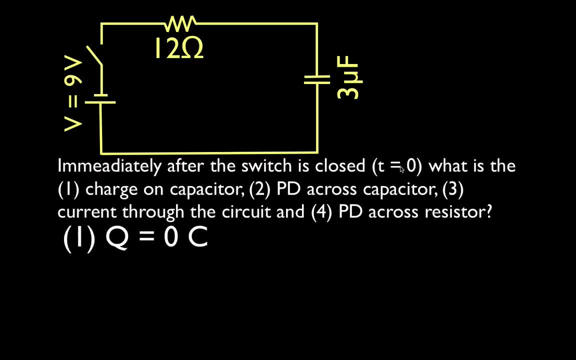 after the switch has been closed, the charge on the capacitor is zero. Nothing has reached the capacitor. Now, if the charge on the capacitor is zero and we know Q equals C times V, if we were to solve for V, we would know then that the voltage- there's no potential. 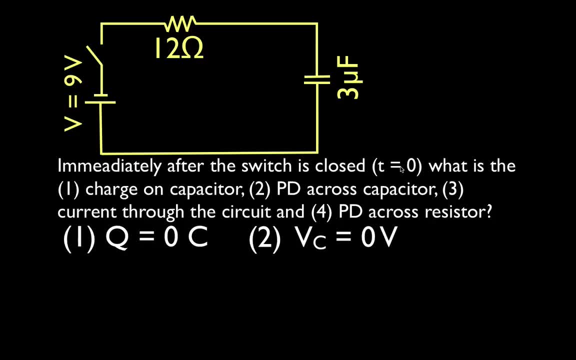 difference across the capacitor: No charge and no potential difference. But the current is actually flowing through the circuit. It's just that none of it has really reached the capacitor yet. The current we're going to use, V equals I times R. We're going to solve: I equals V divided by R. 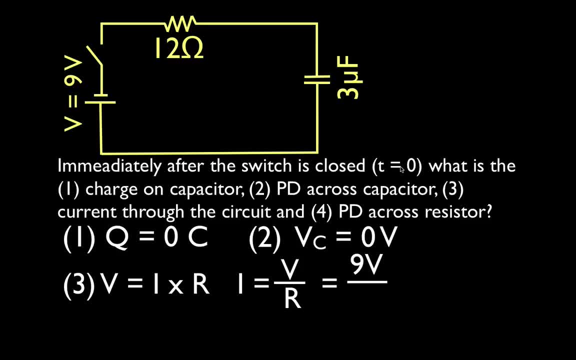 We have a voltage: It's 9 volts. We have a resistance: It's 12 ohms. That means that the current through the circuit is going to reach the capacitor. So we're going to solve: I equals V times R. We're going to solve: I equals V divided by R. We have a voltage: It's 9 volts. We have a. 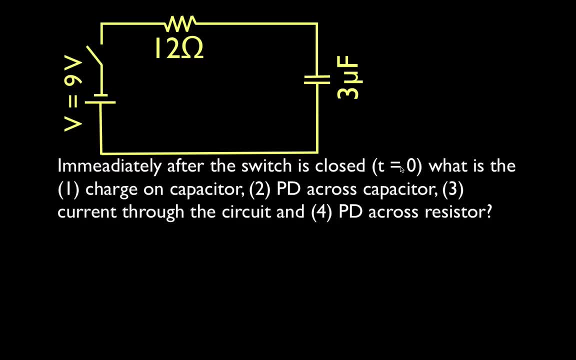 has been closed, which we often call time equals zero. Now, I think of it not really as time equals zero. It's right after the switch has been closed, so it's not really zero, It's a fraction of a second or a very small amount of time. 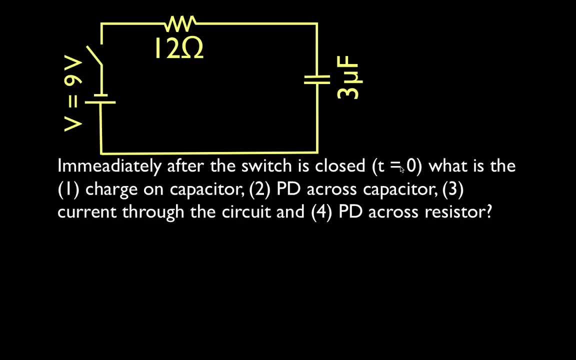 But what happens? what does this circuit look like right after the switch has been closed? We want to know what is the charge on the capacitor, what is the potential difference across the capacitor, what is the current through the circuit and the resistor and 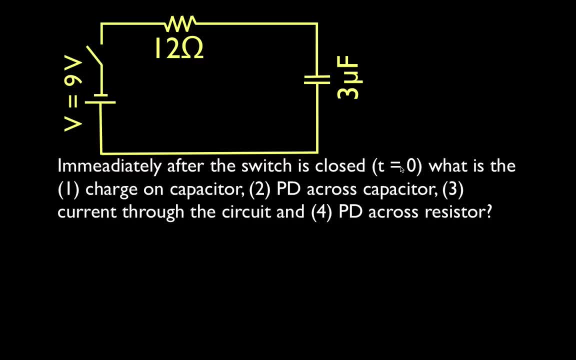 what is the potential difference? or the voltage drop across the resistor. And this is right after the switch has been closed. And this is the way I think about this type of problem: Right after the switch is closed, all of the current, the total amount of current, the 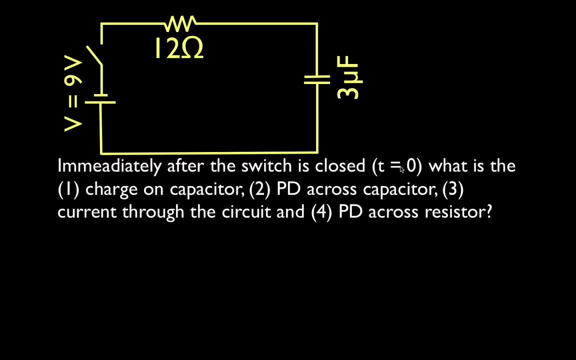 current is flowing through the circuit and the resistor, But none of this current or no charge has yet reached, or no charge has been put onto the capacitor. There is no charge on the capacitor. Okay, None of the charge has reached the capacitor, So really right. 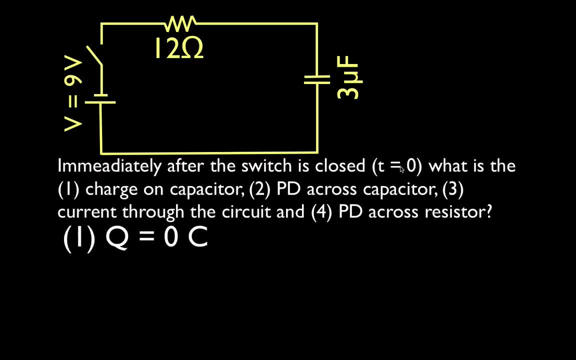 after the switch has been closed, the charge on the capacitor is zero. Nothing has reached the capacitor. Now, if the charge on the capacitor is zero and we know Q equals C times V, if we were to solve for V, we would know then that the voltage- there's no potential. 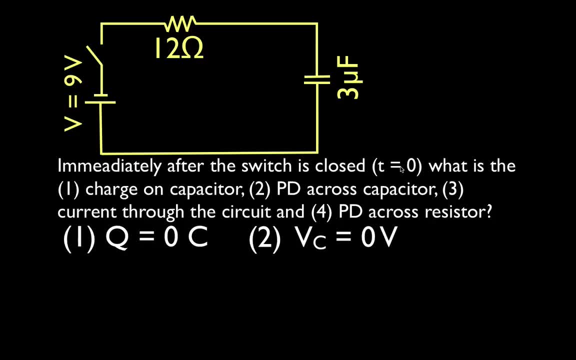 difference across the capacitor: No charge and no potential difference. But the current is actually flowing through the circuit. It's just that none of it has really reached the capacitor yet. The current we're going to use, V equals I times R. We're going to solve: I equals V divided by R. 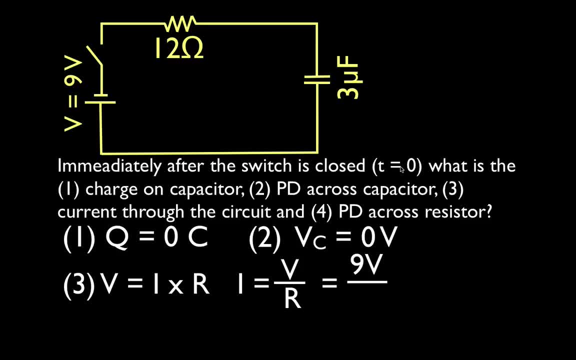 We have a voltage: It's 9 volts. We have a resistance: It's 12 ohms. That means that the current through the circuit is going to reach the capacitor. So we're going to solve: I equals V times R. We're going to solve: I equals V divided by R. We have a voltage: It's 9 volts. We have a. 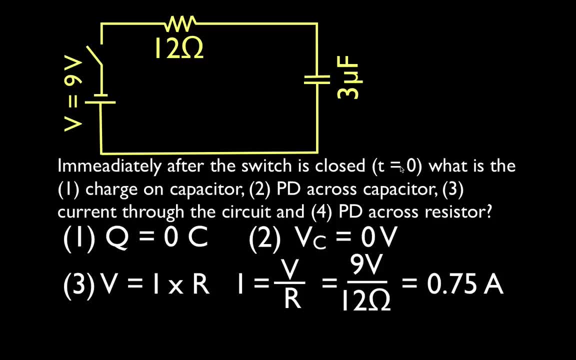 resistance: It's 9 volts. We have a resistance. We have a voltage: It's 9 volts. We have a through. the resistor is 0.75 amps. Okay, We have current, but no charge. Well, where is all the? 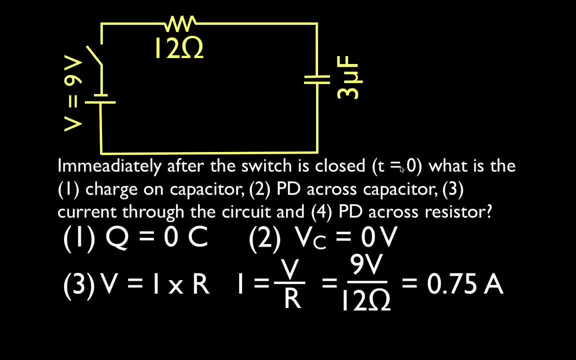 through the resistor is 0.75 amps. Okay, We have current but no charge. Well, where is all the power that's in the circuit? Where not the power? where is all the voltage that's in the circuit? Well, it's on the resistor And the voltage is equal to the current. 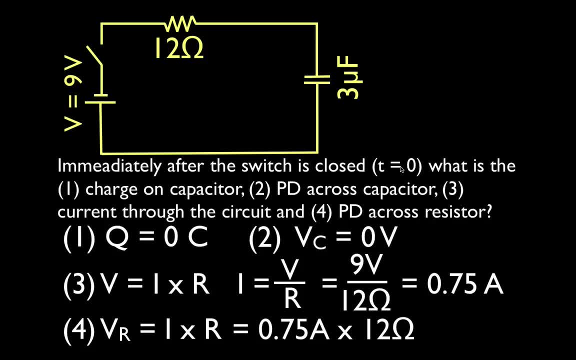 times the resistance, And that means that the voltage is equal to 0.75.. We figured out earlier. that's the current. That current is flowing through the resistor. That's the only thing that's using any of that energy or any of that voltage. And so we're going to solve: I equals V. 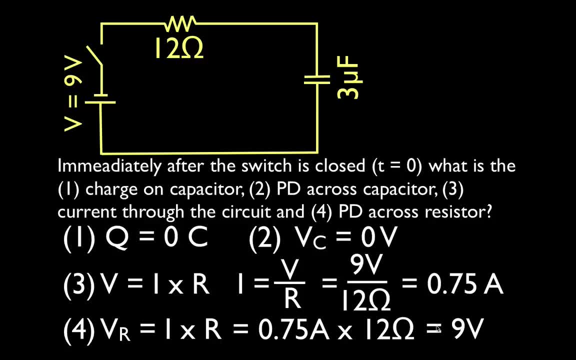 and therefore we have that. we have nine volts, and that should match the battery. okay, nine volts, all of it is on the resistor, none of it is on the capacitor yet. okay, so pretty straightforward. now we're going to talk about time equals infinity, or, after a long time, what is the? 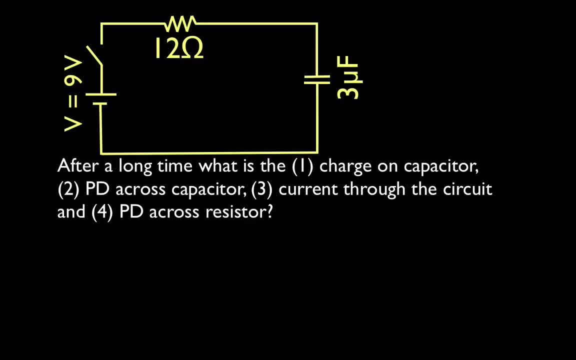 charge on the capacitor. what is the potential difference across the capacitor, what is the current through the circuit and what is the potential difference across the resistor? now, the key here is: after a long time the capacitor is fully charged. that's basically what they mean when they say after a long time the capacitor is fully charged and when the capacitor is fully. 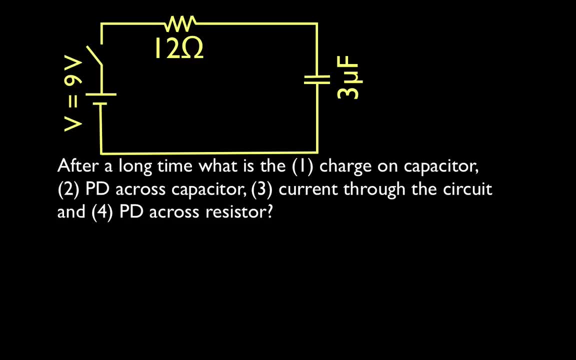 charged, there is no current flowing through the circuit. that's the key. on the previous slide we had current but no charge. now we have charge but no current, all right. so i'm going to answer these not in one. two, three. you order. we're going to do number three first, after the capacitor is charged after a long time. 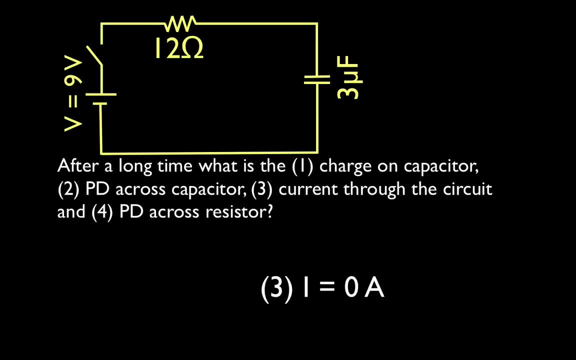 there's no current flowing in the circuit anymore. so therefore the current is zero amps. and if there's no current flowing through the circuit, we can do v equals i times r, v equals i times r, i equals zero. so that means that v is equal to zero, so there's no current. 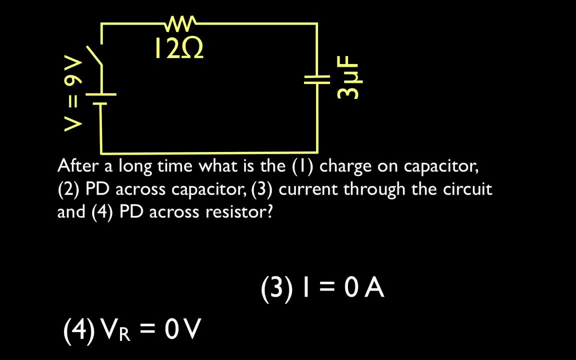 flowing through the circuit. there's no voltage across the resistor. no voltage drop. well, where is all that voltage? the voltage is now on the capacitor. at time equals infinity. at time equals a long time. the voltage is on the capacitor. the voltage of the capacitor is equal to the voltage of the battery. 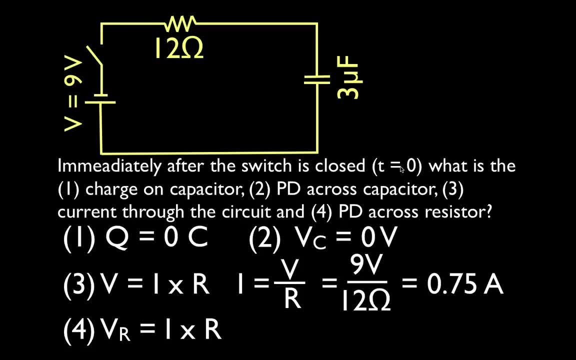 power. that's in the circuit. Where not the power? but where is all the voltage that's in the circuit? Well, it's on the resistor and the voltage is equal to the current times. the resistance, and that means that the voltage is equal to 0.75.. We figured out earlier. that's the current. 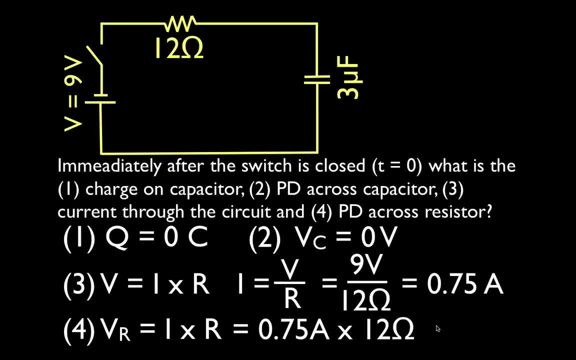 That current is flowing through the resistor. That's the only thing that's using any of that energy or any of that voltage, and therefore we have that. we have nine volts and that should match the battery. okay, nine volts, all of it is on the resistor, none of it is on the capacitor yet. okay, so pretty straightforward. 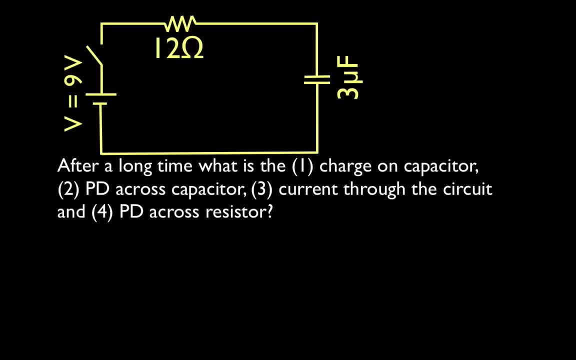 now we're going to talk about time equals infinity, or, after a long time, what is the charge on the capacitor, what is the potential difference across the capacitor, what is the current through the circuit and what is the potential difference across the resistor? now, the key here is: after a long time, the capacitor is fully charged. that's basically what they mean. 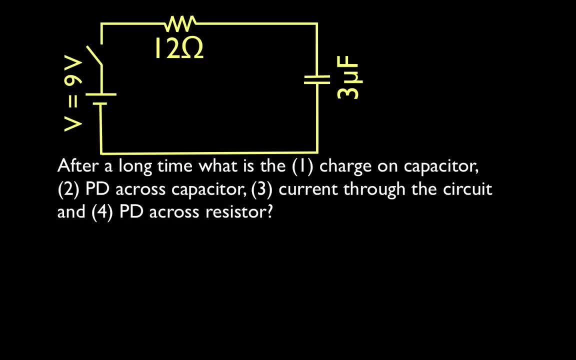 when they say after a long time the capacitor is fully charged. and when the capacitor is fully charged, there is no current flowing through the circuit. that's the key. on the previous slide we had current but no charge. now we have charge but no current. all right, so i'm going to answer these. 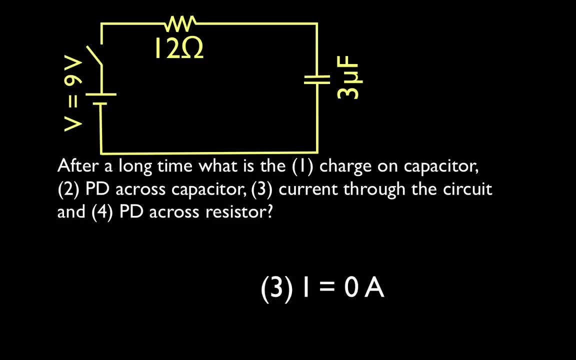 not in one, two, three, you order. we're going to do number three first. after the capacitor is charged, after a long time there's no current flowing in the circuit anymore. so therefore the current is zero amps and if there's no current flowing through the circuit, we can do: v equals i times r. 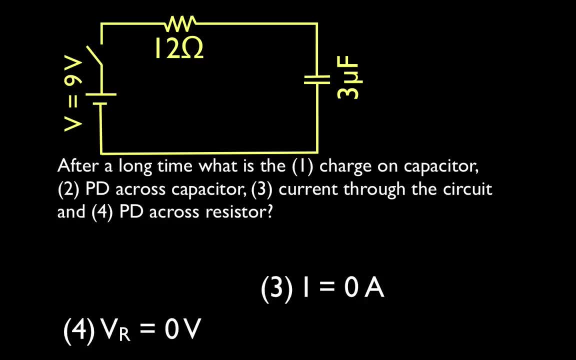 v equals i times r, i equals zero. so that means that v is equal to zero. so there's no current flowing through the circuit, there's no voltage across the resistor, no voltage drop. well, where is all that voltage? the voltage is now on the capacitor. at time equals infinity. at time equals a long time. 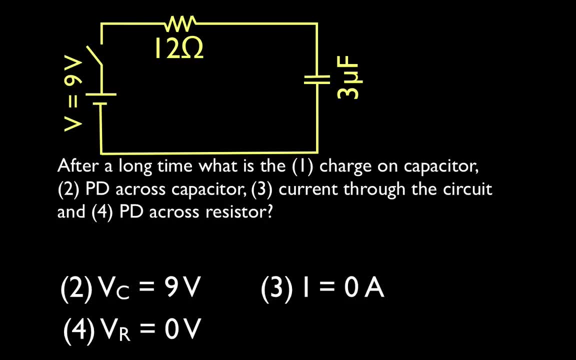 the voltage is on the capacitor. the voltage of the capacitor is equal to the voltage of the battery. all right now we can solve for the charge. how much charge is there? because all the charge is there. we've put all the charge on the capacitor. q equals c times v. we have a three microfarad. 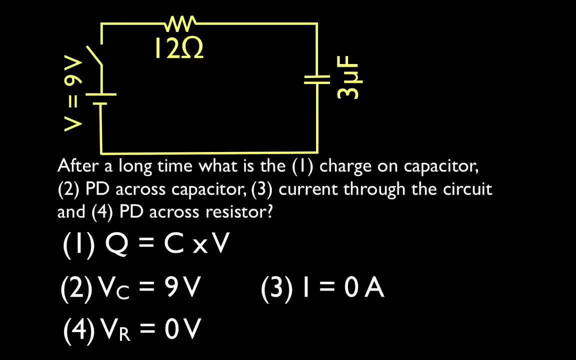 all, right now we can solve for the charge. how much charge is there? because all the charge is there. we've put all the charge on the capacitor. q equals c times v. we have a three microfarad capacitor. we said after a long time the charge, excuse me, the voltage of the capacitor is equal. 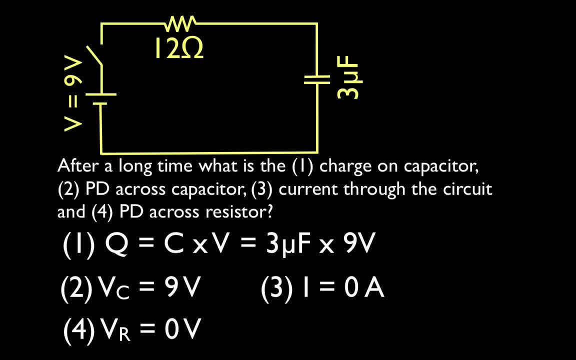 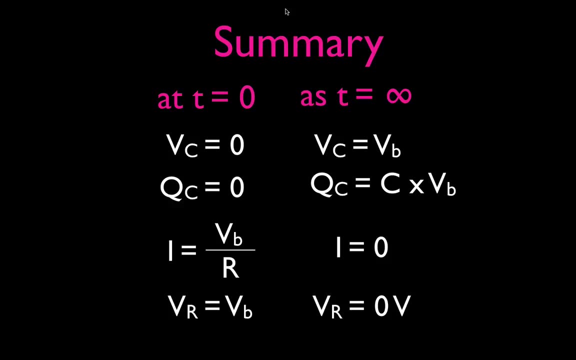 to the voltage of the battery, in this case nine volts. so it's three times nine, twenty-seven micro coulombs. okay, that is after a long time, after time equals infinity. okay. so those are the two cases. i'm just going to summarize them right here. and we have a time equals zero right after. 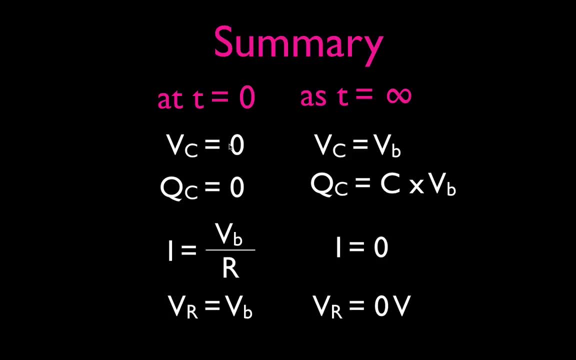 the switch is closed, the voltage on the capacitor is zero, the charge on the capacitor is zero, the current is equal to the voltage of the battery. times the total resistance. in this case we just had one resistor, and the voltage of the resistor is equal to the voltage of the battery. now, after 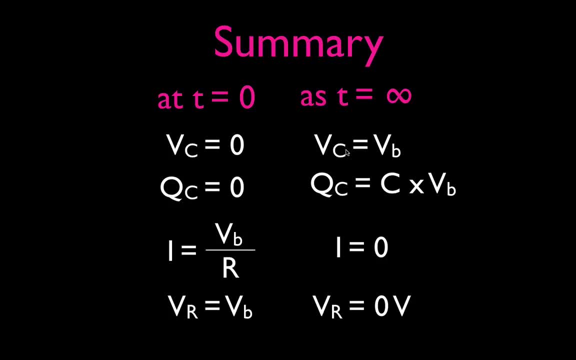 a long time. it's kind of the opposite. the voltage of the capacitor is equal to the voltage of the battery. now we have charge, we're going to. we would solve that by using q equals c times v. q equals capacitance times the voltage of the battery. okay. 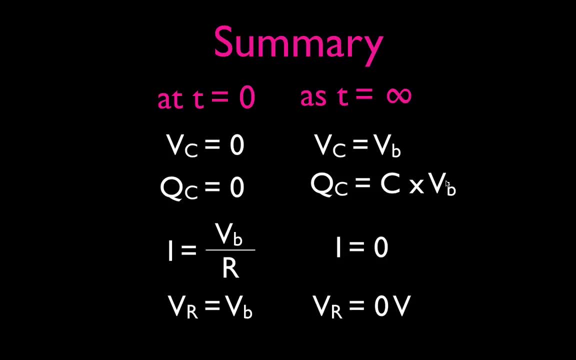 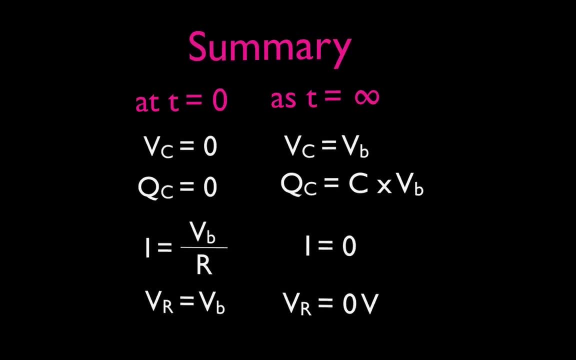 because all the charge is now on the capacitor, there's no current and the voltage across the resistor is zero. all right now one more thing before we finish. i just want to show you these quick curves. these are often curves that are used for rc circuits. i'm not going to go into a lot of 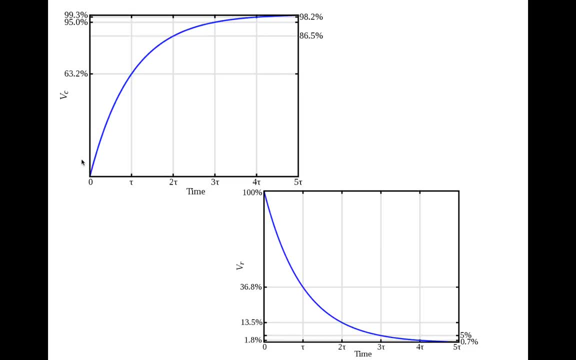 detail, but you'll notice, this is the voltage of the capacitor. this is that. this is over time. now. okay, this is time down here. this is the voltage of the capacitor. this is just time. this is tau. this is the time constants one, time constant two, and this is the voltage of the capacitor. 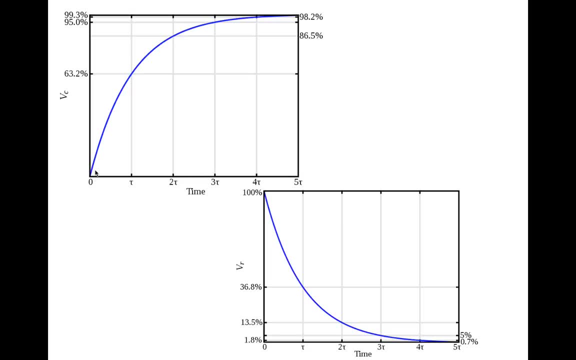 which we didn't talk about. but just realize time is increasing, okay, and the voltage here is increasing and you can see, over time the voltage on the capacitor goes from zero to one hundred of the battery and the here, this one is the same thing, time down here, voltage of the resistors. so 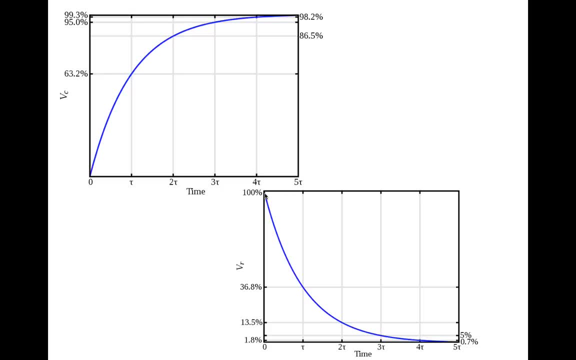 over time. the voltage on the resistor is the greatest. in our case it was nine, and then it goes down to zero volts. in this case, here it was zero volts, Zero volts, Zero volts. One name is- I'm scared, but it works- would go up to nine. here it's shown in percentages. 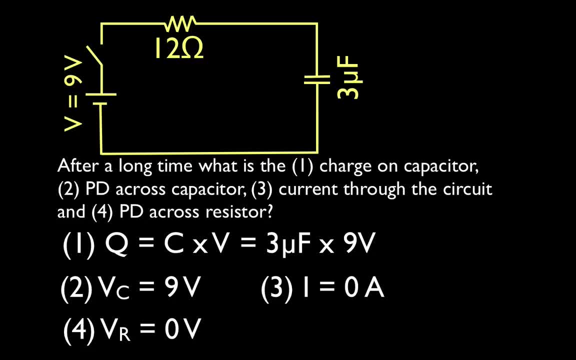 capacitor. we said after a long time, the charge, excuse me, the voltage of the capacitor is equal to the voltage of the battery, in this case nine volts. so it's three times nine, twenty-seven micro coulombs. okay, that is after a long time. after time equals infinity, okay, so those are the. 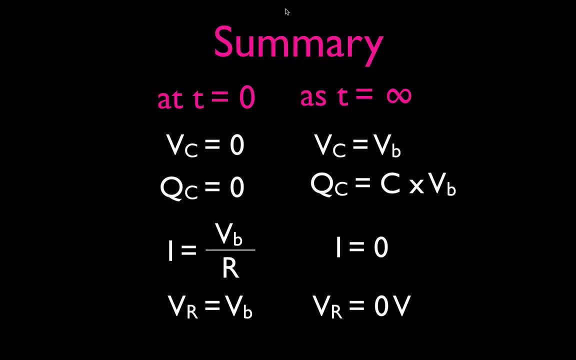 two cases. i'm just going to summarize them right here. and we have a time equals zero. right after the switch is closed, the voltage on the capacitor is zero, the charge on the capacitor is zero, the current is equal to the voltage of the battery times, the total resistance in this case. we just 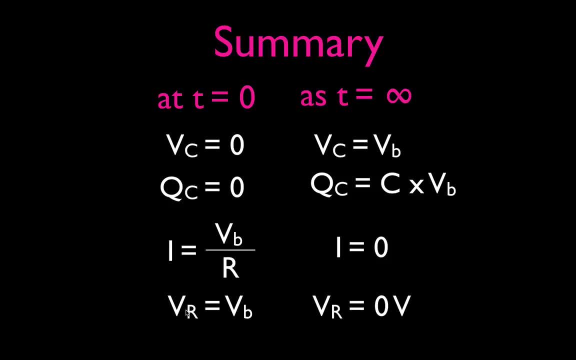 had one resistor and the voltage of the resistor is equal to the voltage of the battery. now, after a long time, it's kind of the opposite. the voltage of the capacitor is equal to the voltage of the battery. now we have charge, we're going to. we would solve that by using q equals c times v. 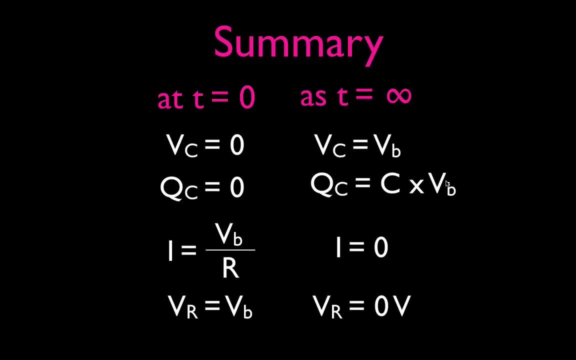 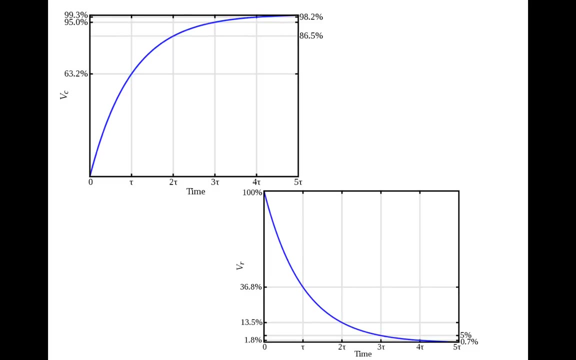 q equals capacitance times the voltage of the battery. okay, because all the charge is now on the capacitor, there's no current and the voltage across the resistor is zero. all right now. one more thing. before we finish, i just want to show you these quick curves. these are often curves that are used for rc circuits. i'm not going to go into a lot of. 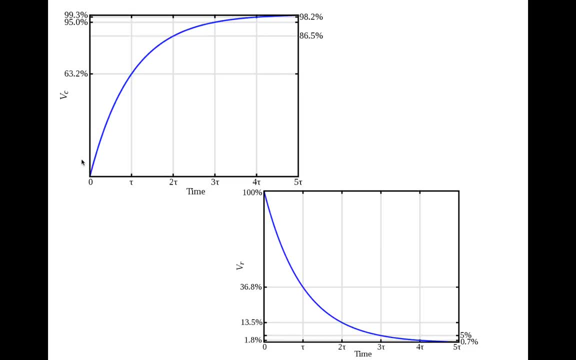 detail, but you'll notice, this is the voltage of the capacitor. this is that. this is over time. now. okay, this is time down here. this is the voltage of the capacitor. this is just time. this is tau. this is the time constants one, time constant two, and this is the voltage of the capacitor. 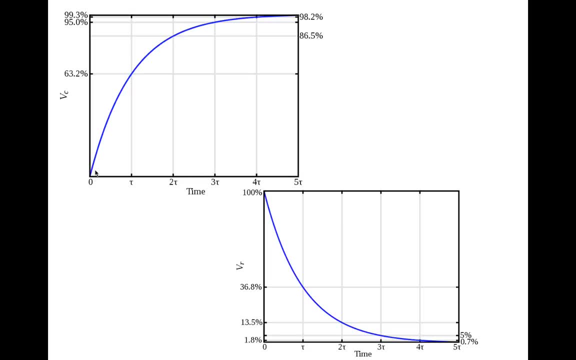 which we didn't talk about. but just realize time is increasing. okay, and the voltage here is increasing and you can see, over time the voltage on the capacitor goes from zero to 100 of the battery and the here, this one is the same thing, time down here, voltage of the resistor, so over 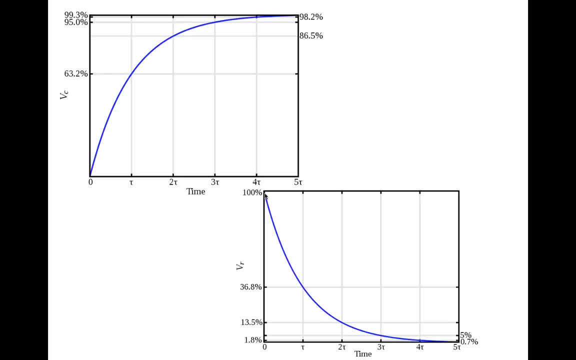 time the voltage on the resistor is the greatest- in our case it was nine- and then it goes down to zero volts. in this case, here it was zero volts and it go up to nine. here it's shown in percentages. okay, so that's how rc, that's, in general, how rc.